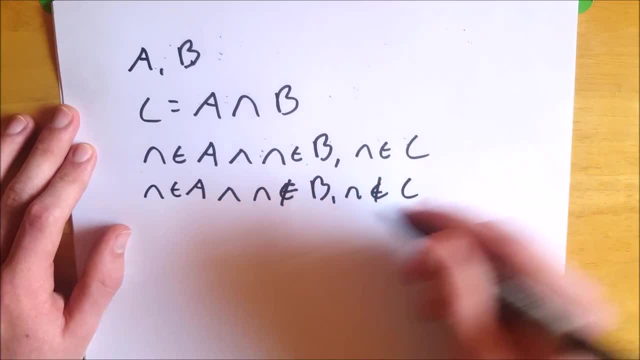 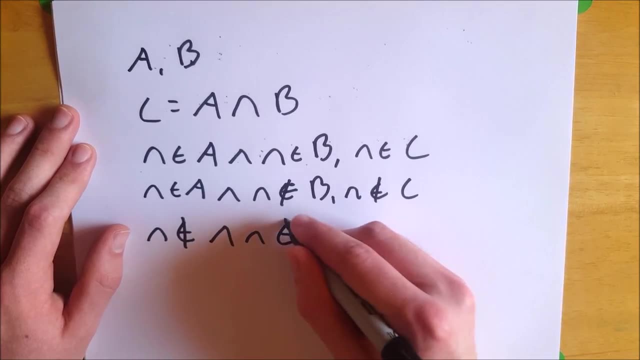 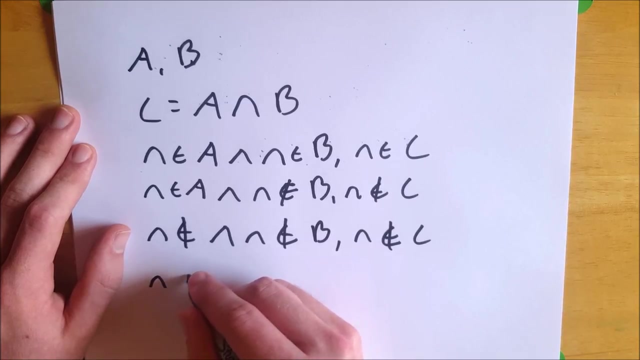 then N is an element of B, Then if N is not an element of C, then if N is not an element of A and N is not an element of B, then N is not an element of C. And lastly, if N is not an element of A and N is an element of B, then still N is not an element of C. 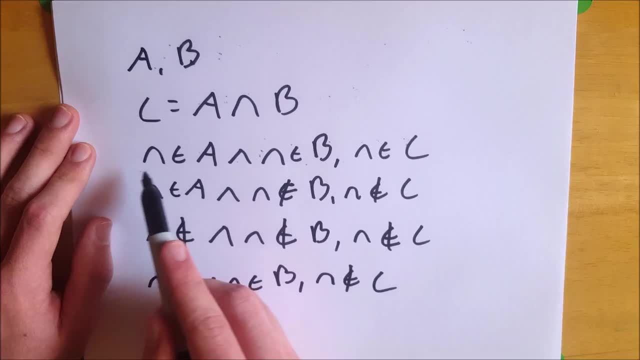 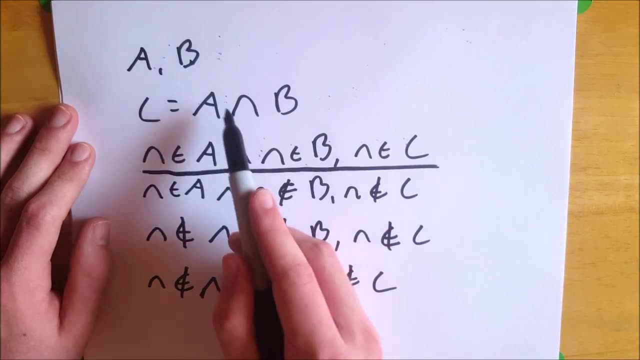 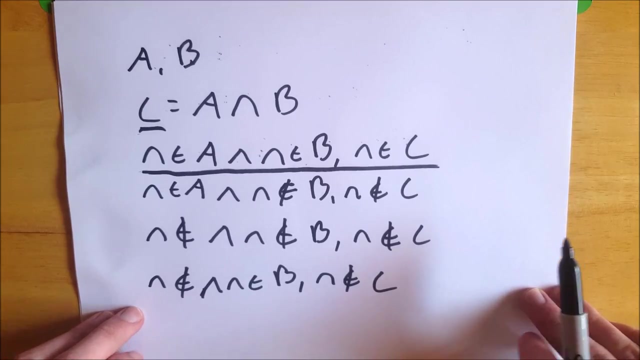 So you can see, the only case here that results in N being an element of C is this one here, where n is both in a and n is in b. So if an element is in both a and b, then it will be in their intersection c. So let's just go over a quick example and that will be it for this video. 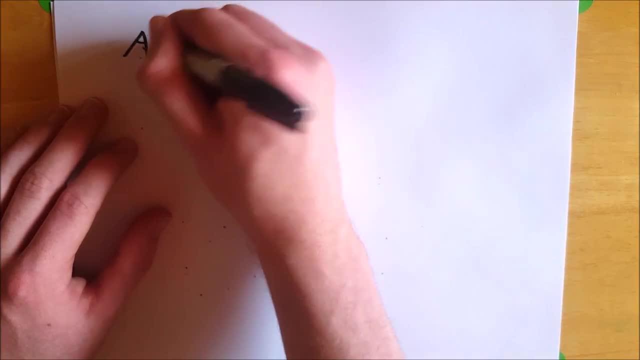 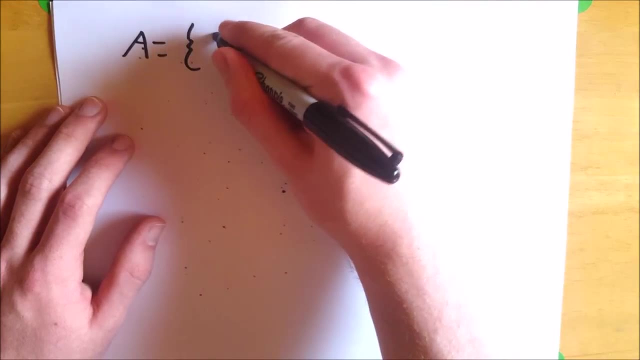 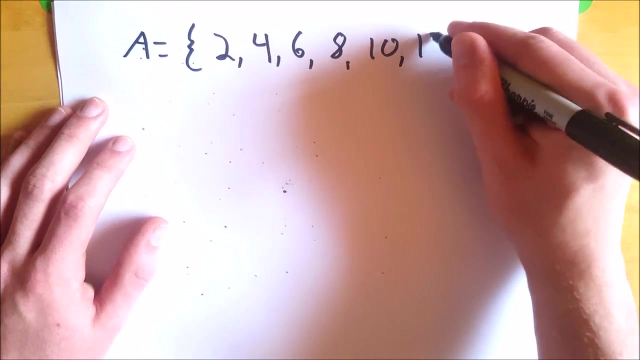 So let's say, set a is equal to all positive even numbers less than or equal to 12.. So that would mean that a is the set containing 2, 4, 6, 8, 10 and 12, because I said less than or equal to. Let's: 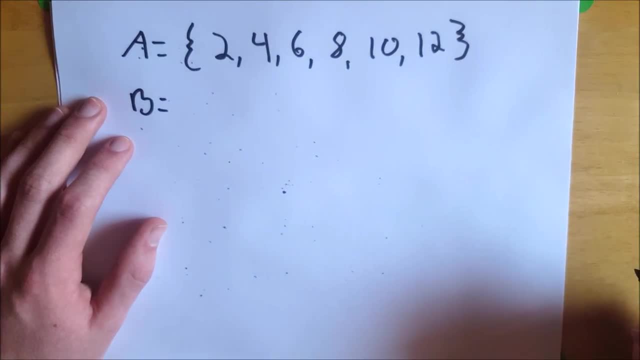 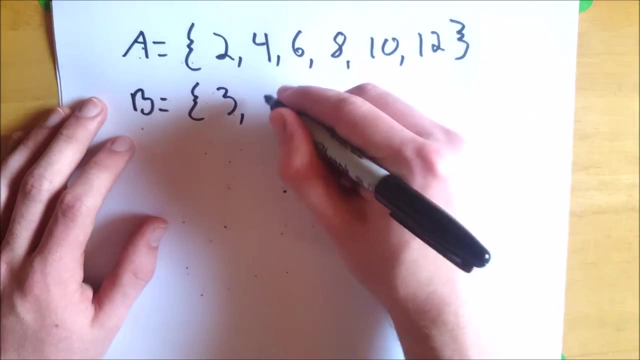 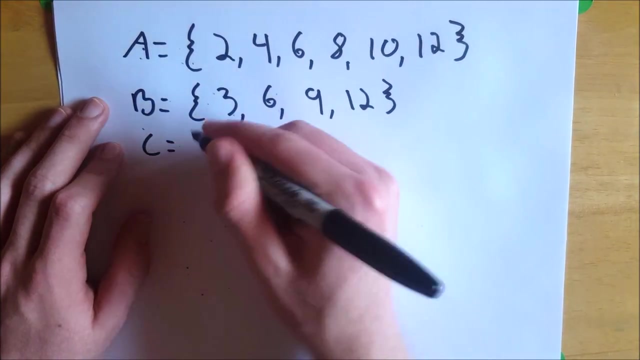 define b has being the set containing all positive multiples of 3 that are less than or equal to 12.. So it starts with 3, 6, 9 and again ending with 12.. And now we want to find c, which is a, and we'll suffice it out to be c, which is c. If we write a set of positive or 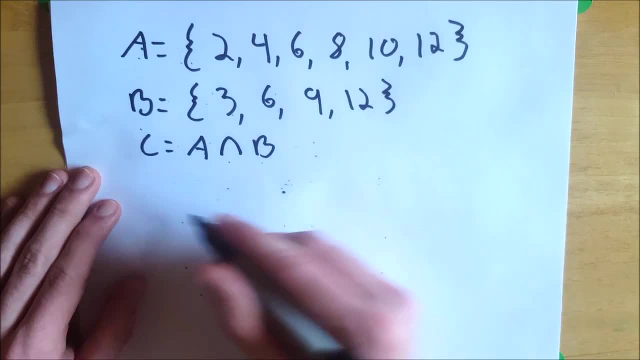 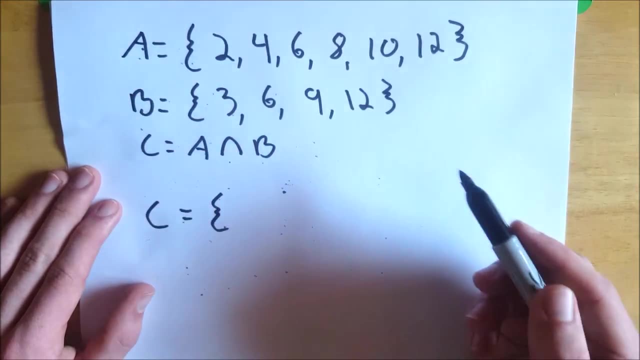 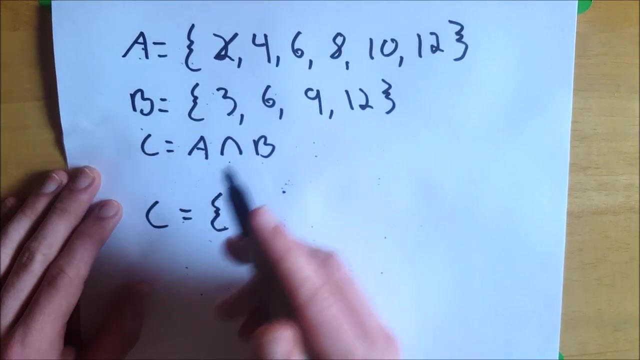 intersect B. So what is C? Well, let's use the rules that we just went over and figure it out. Open up the set. Is it going to contain 2? No, it won't, because 2 is in A but it is not in B. What about 4?? 4 is in A but it's not in B, so 4. 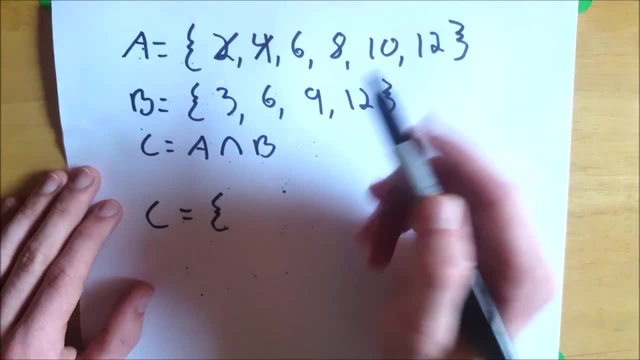 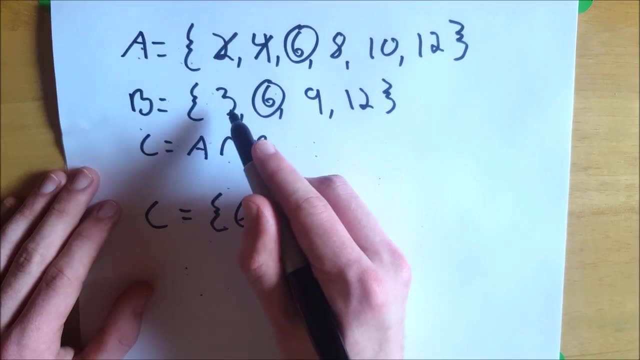 will not be in our intersection either. What about 6?? 6 is in A and 6 is in B, so 6 will be in C. Let's jump back to 3 here, Not in A, so it's not gonna cut it. 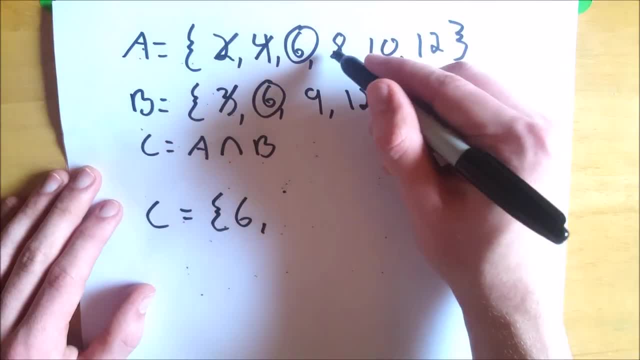 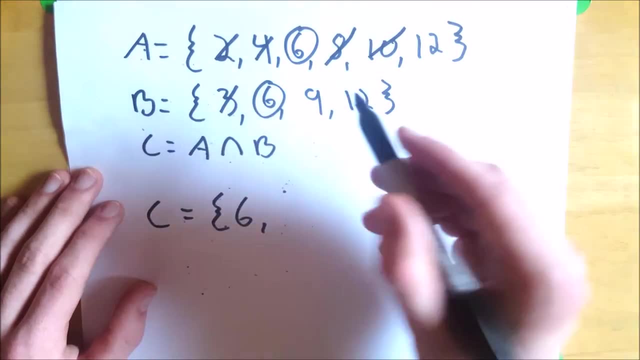 8, not in B. It is in A, but it isn't in B, so we won't include 8 either. What about 10?? 10 is in A, but it's not in B, so we will not include it. 9 is in B, but. 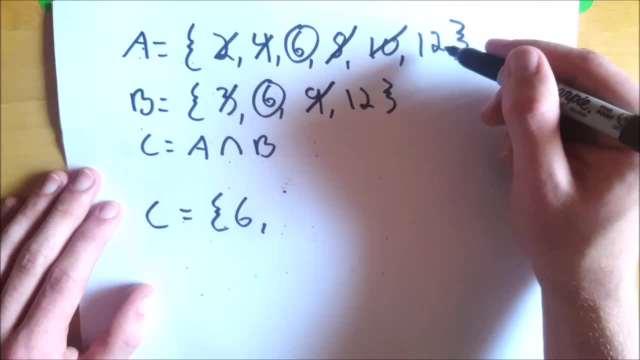 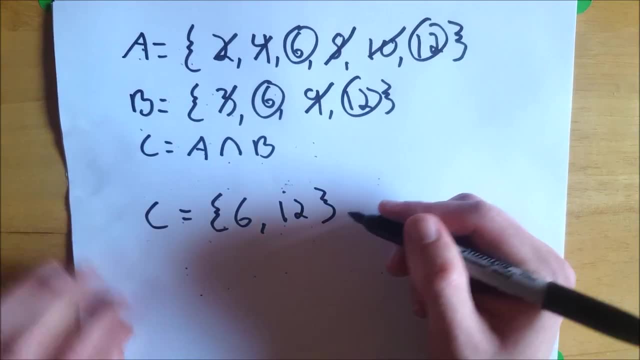 not in A, So we will not include that. And then, lastly, 12 is in A and it is in B, So that will be the final element in our tiny little set. So you see, it's in first place. Now let's see the other two pieces of the set. So we'll